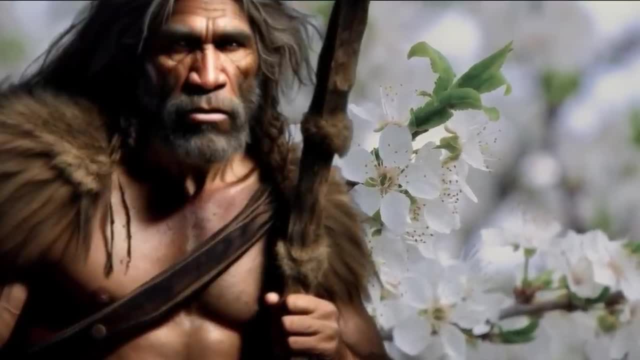 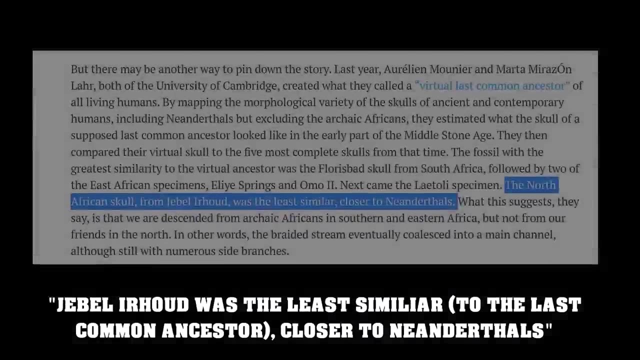 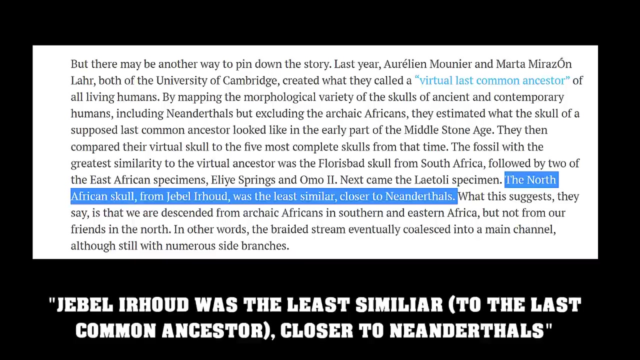 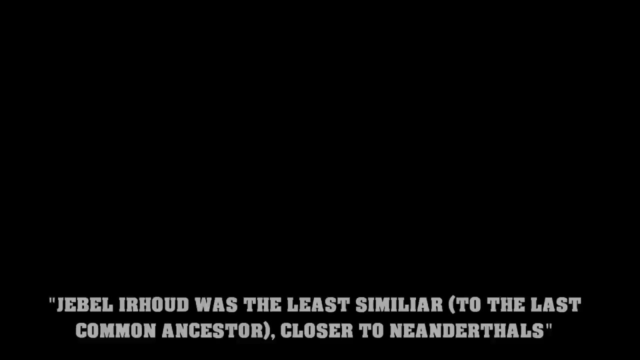 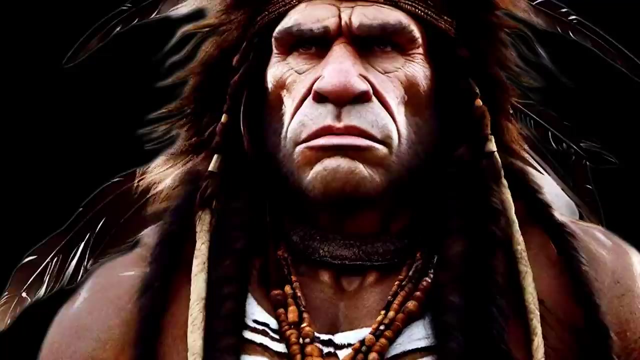 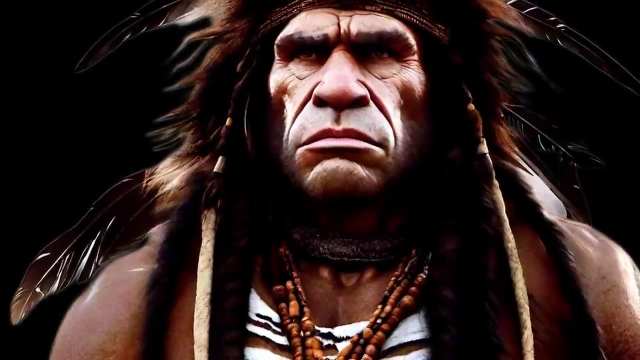 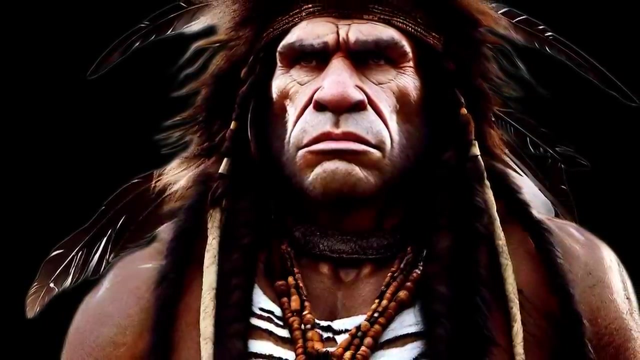 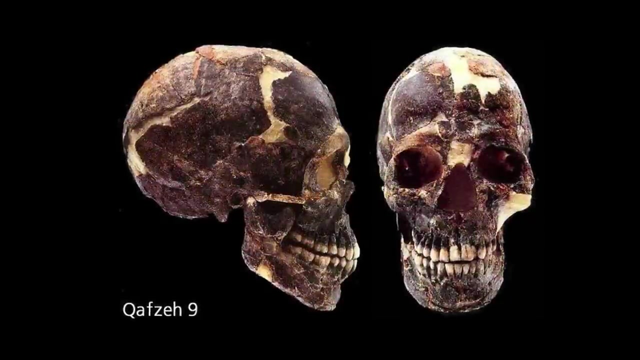 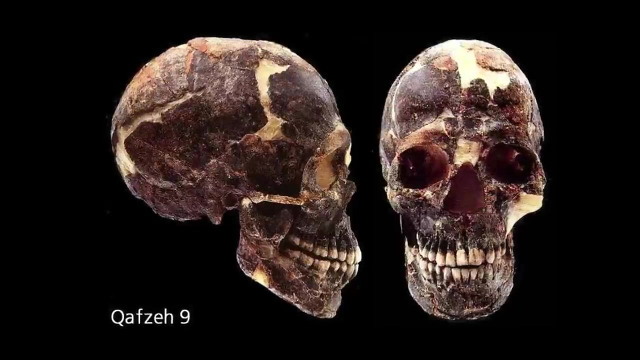 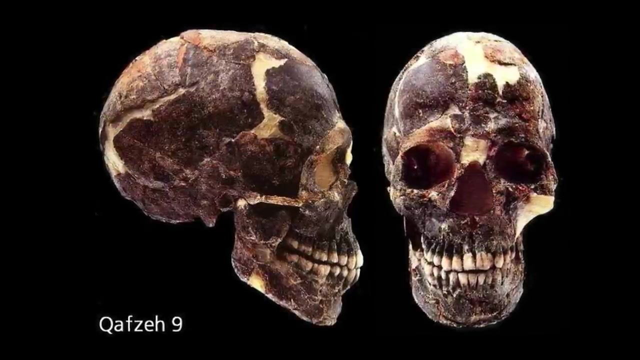 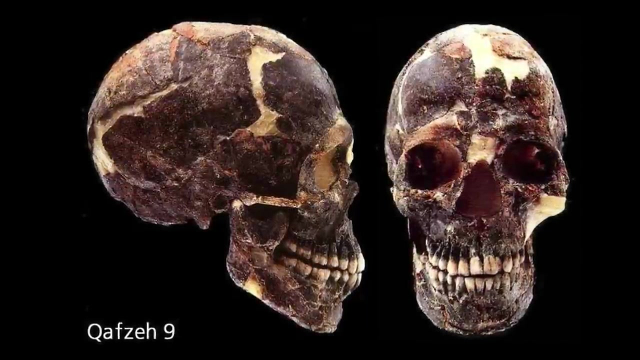 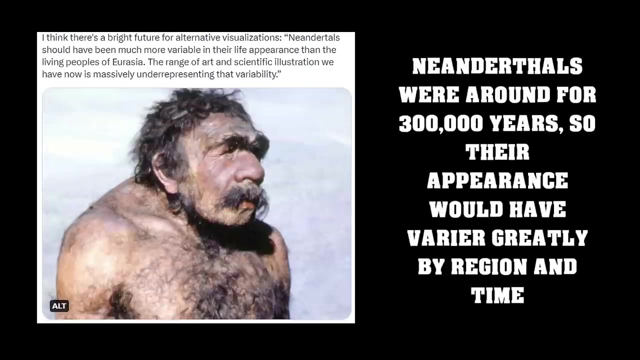 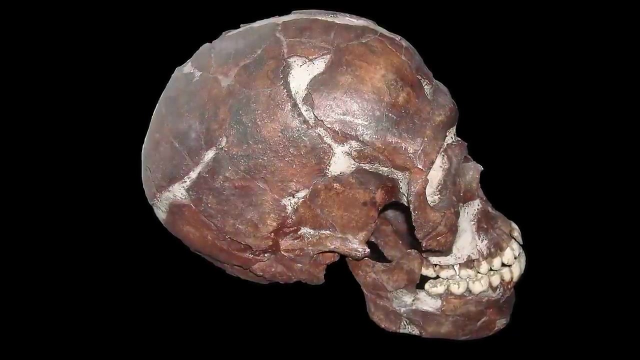 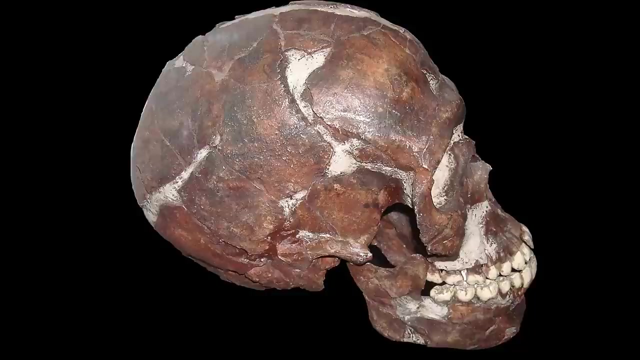 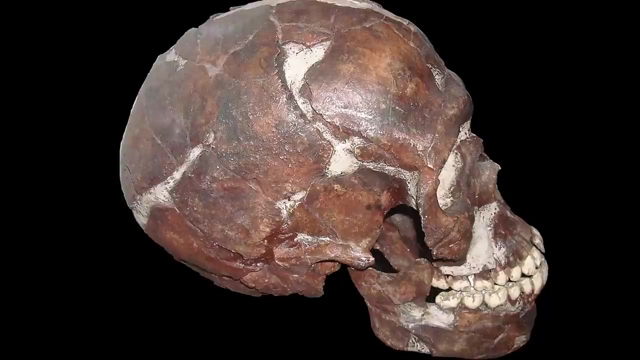 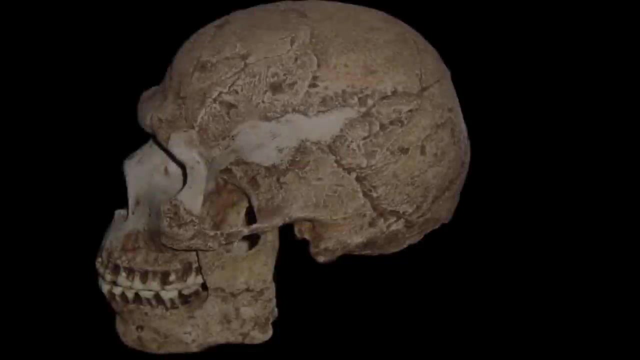 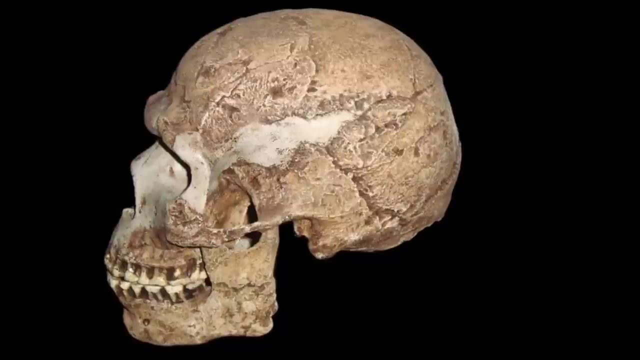 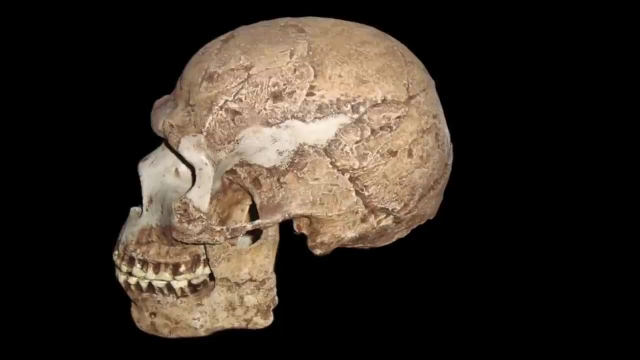 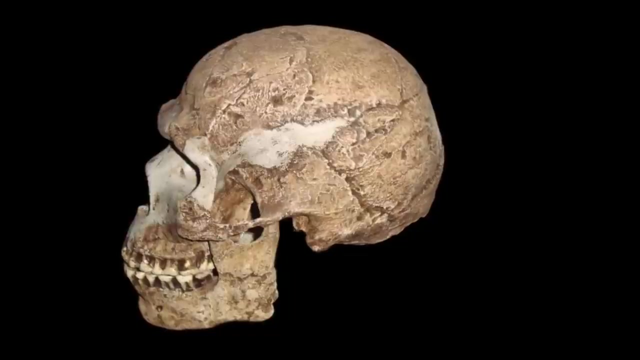 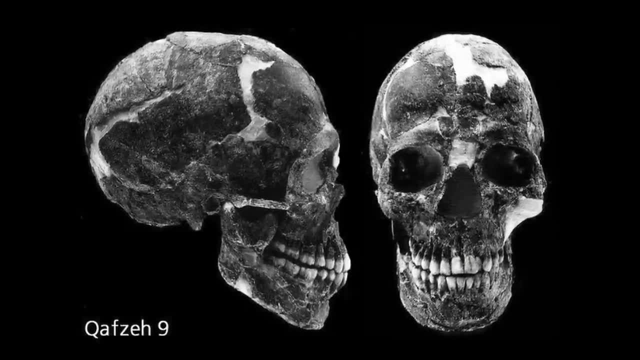 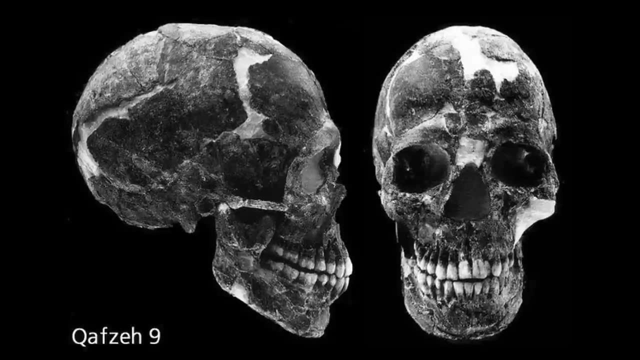 were not as intelligent as us. there is evidence that they practiced chemistry, buried their dead and even created art: The intentional burial of the dead, the presence of grave goods and the arrangement of bodies in certain ways which may suggest ritualistic practices. 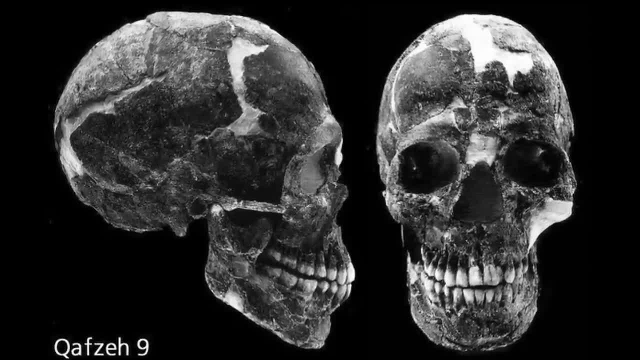 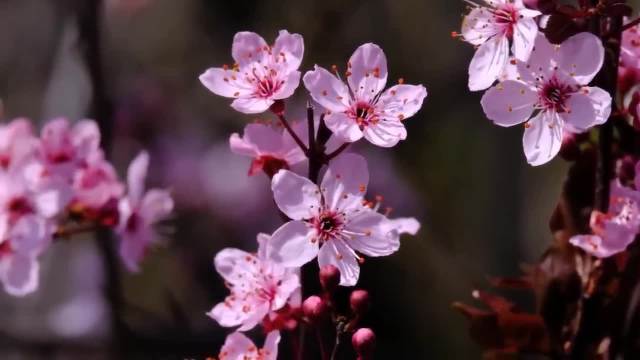 all lend support to this theory. In Spain, evidence for a 50,000-year-old Neanderthal burial ground has been discovered, including the remains of at least three individuals. The arrangement of remains at the burial site suggests that Neanderthals may have performed.